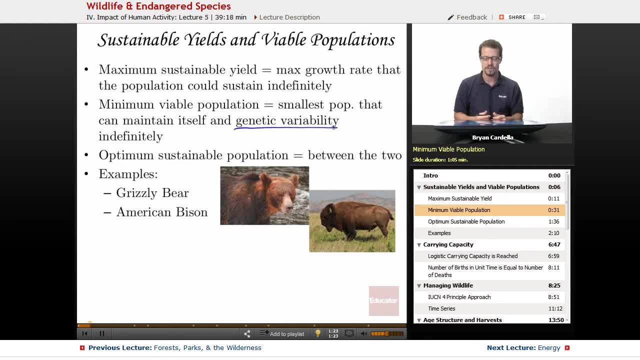 that's desirable in the long term for a population, They'll be extremely vulnerable to environmental change, more so than if you had a lot more than two. So the maximum sustainable yield and minimum viable population is going to vary depending on the organism we're. 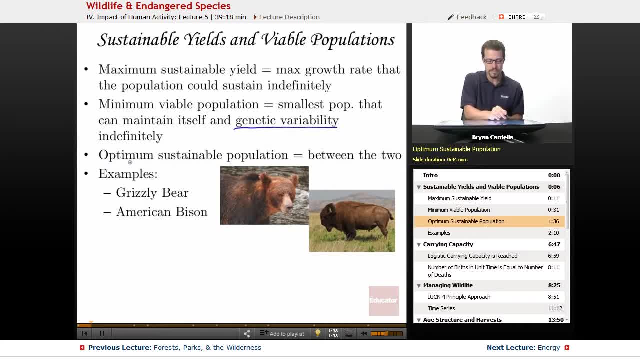 talking about In between those two is the optimum sustainable population. So it's between the two. It's that, in a sense, happy medium. It's not reasonable, especially if a species is threatened or endangered, to get up to the maximum sustainable yield. That may not be feasible. 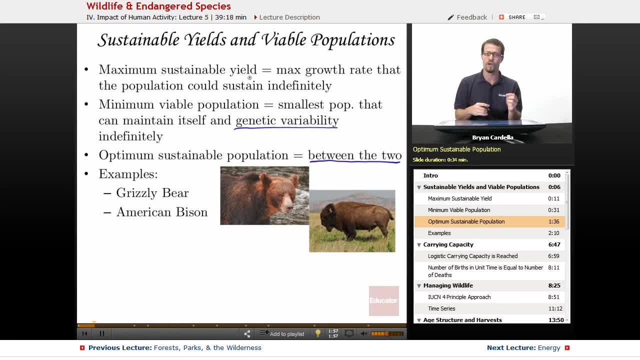 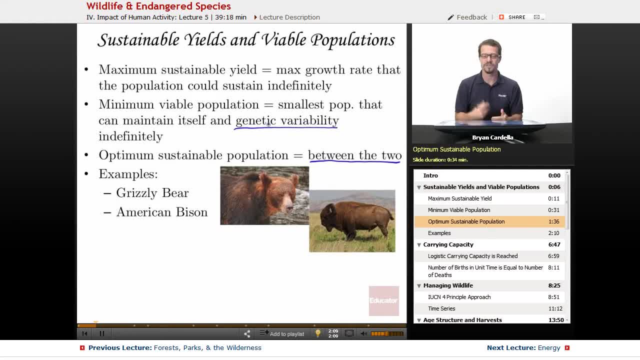 optimum in the middle is what a lot of scientists or environmentalists are shooting for. Here's some examples with the grizzly bear and the American bison. The grizzly bear is fascinating to me. I live in California. It's on the state flag. 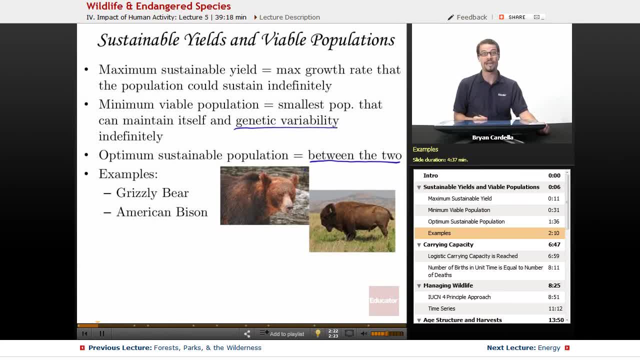 but there are no grizzly bears in California anymore. There used to be a lot of them in the United States. Not so much anymore. You have to go up into Canada for a good chance of seeing a grizzly bear, So they are definitely endangered. 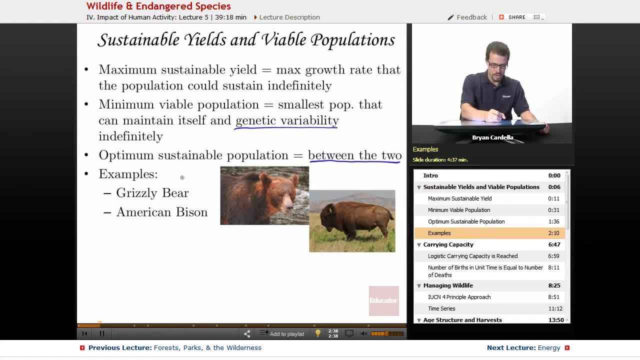 And some little facts about the grizzly bear. When you're looking at the females, you're seeing adults up to about 300 pounds, And then with males up to about 600 pounds, A full-grown one standing up on its hind legs, eight feet tall. That's pretty intimidating. 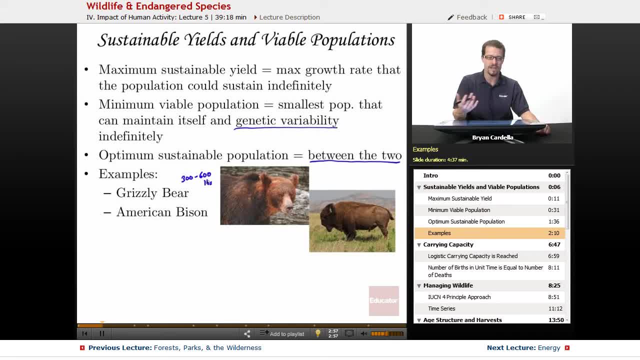 So, yeah, part of the reason they are endangered is, well, they were considered a threat And a lot of them were hunted for and killed more so than probably should have, And that's why we don't see them as much in the United States. 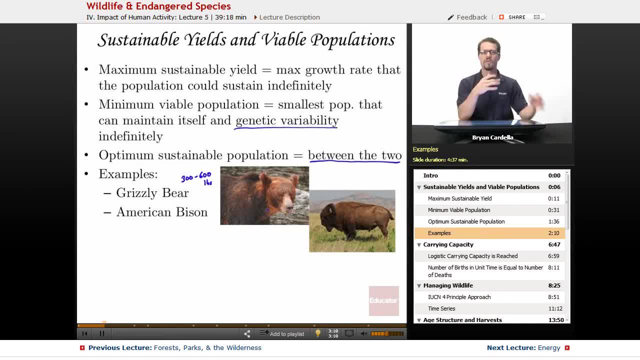 So how can we estimate where the grizzly population was If we go back to the 1800s? we don't have a time machine, obviously, but in terms of records that were kept, we don't have exact numbers And they wouldn't have been able to give us exact numbers back then. 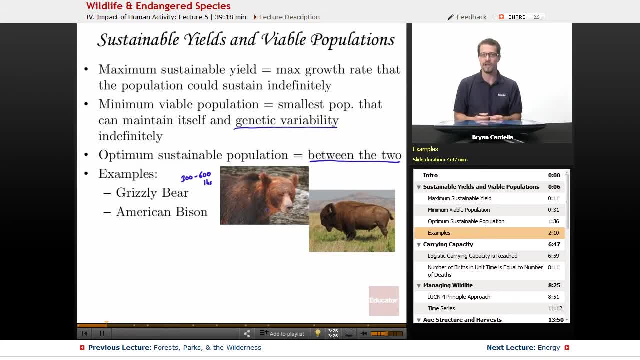 But we can look at Lewis and Clark's expedition. So in the 19th century, in the early 1800s, when they made that expedition to the West Coast, they kept track of how many grizzly bears they saw, And they were actually very specific. 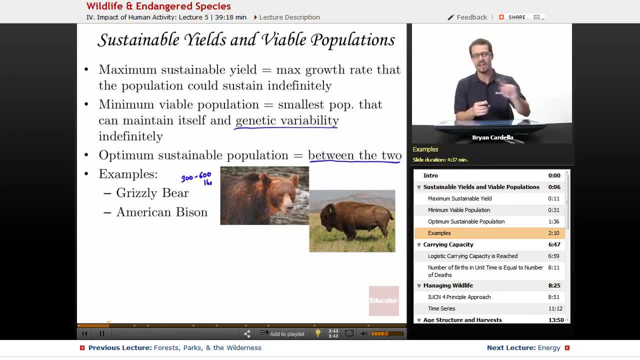 When they passed buffalo or bison, they would just say, oh, there's a lot of them over there, Because they weren't as much of a threat They didn't care to figure out. are there 1,000 bison, Are there 5,000?? They just would say there's a lot of them, But with grizzly bears. 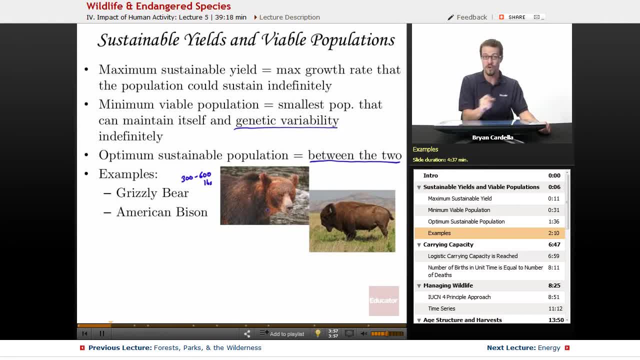 being surprised by seeing one and the potential threat they made note in their journal. we saw a lot of grizzly bears today. We saw three of them today And when you add up the total number, in their journey they encountered 37- over 1,000 miles that they traveled. 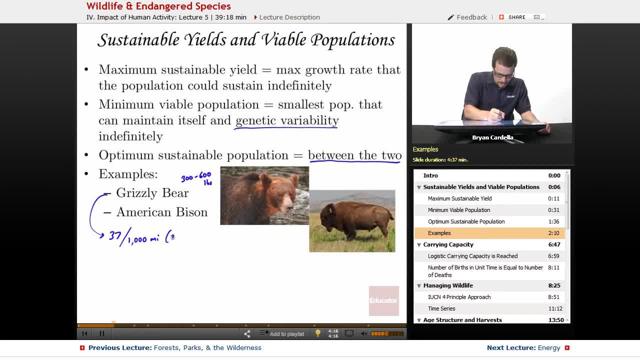 They kept miles in their journal rather than kilometers, And so that comes down to about 3.7 grizzly bears per 100 square miles of area, And if you consider how many grizzly bears existed back then, they've come up with a calculation that in the early 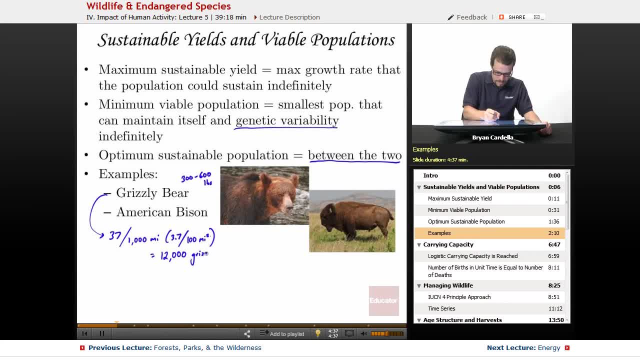 1800s there were about 12,000 grizzly bears. There are significantly less now, But they are protected And hopefully, because of human intervention and regulation in terms of preserving them, we can get back to a reasonable number. 12,000 grizzly bears may not be reasonable. 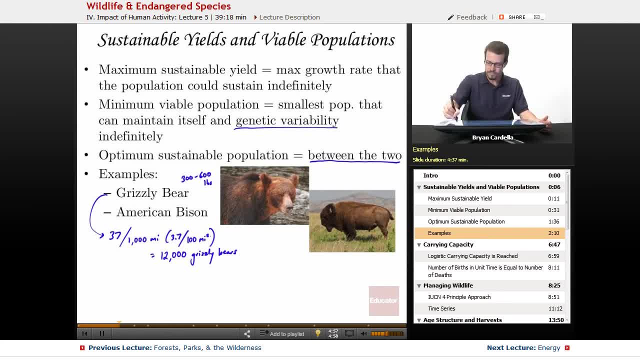 at this point in time. When we look at the American bison- a slightly different tale- We've been able to bring back the American bison to fairly high levels in terms of their overall population numbers. We're certainly not at the maximum sustainable yield. We're not going to go there again. 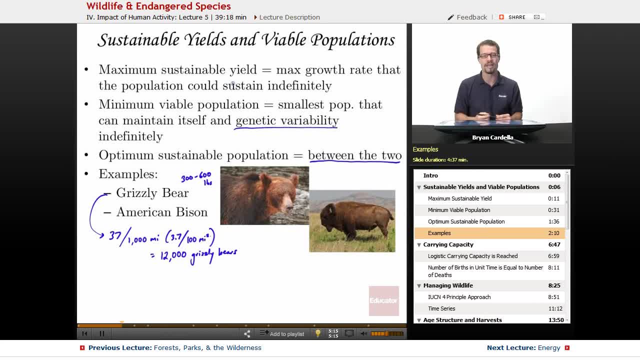 Because in the mid-1800s we're talking millions, millions of bison roaming the plains. A lot of Native American tribes depended on them directly And during especially the middle of the 1800s into the 1870s, a lot of bison were hunted by white Americans And actually a lot of areas were. 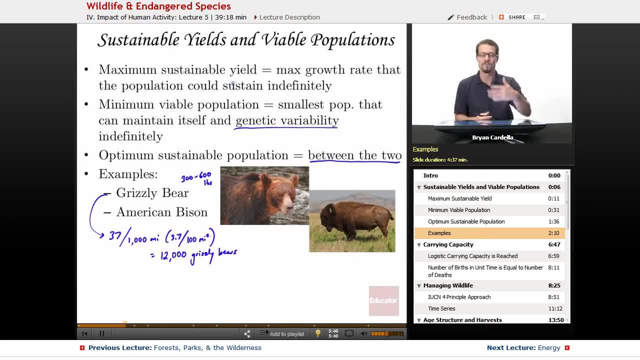 burned to get the Native Americans to move and to get the bison to move. And a lot of bison were killed in that process as well and skinned for hides et cetera. Now the American bison is estimated to be: